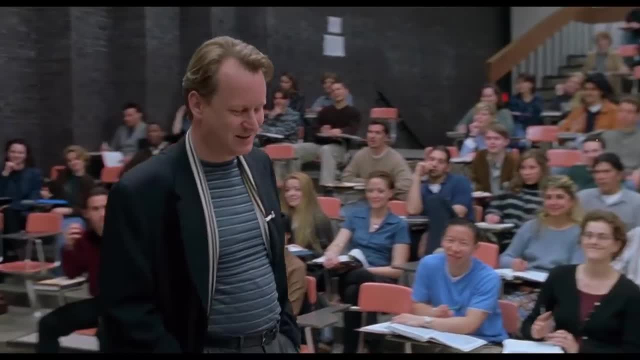 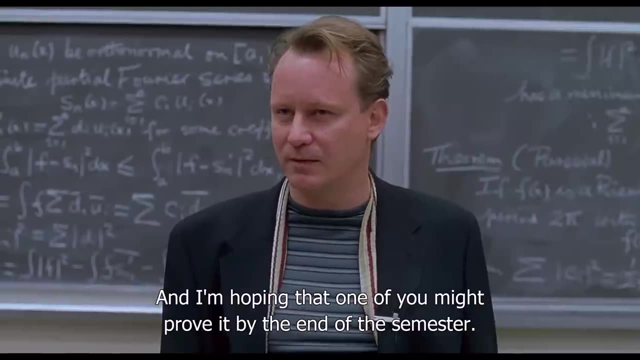 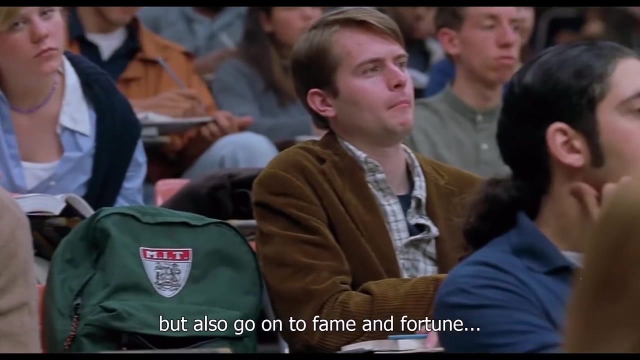 Steven, I also put an advanced Fourier system on the main hallway chalkboard and I'm hoping that one of you might prove it by the end of the semester, And the person to do so will not only be in my good graces but also go on to fame and fortune by having their accomplishment recorded and their name printed in the auspicious MIT Tech. 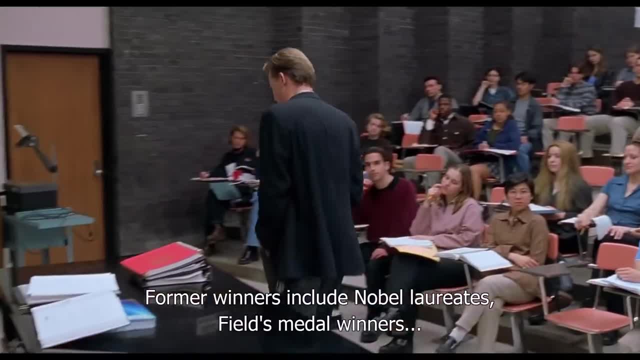 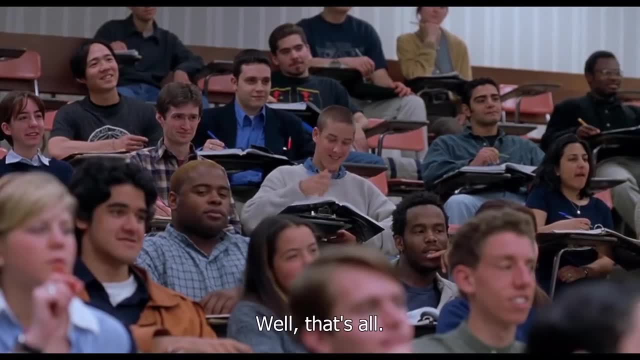 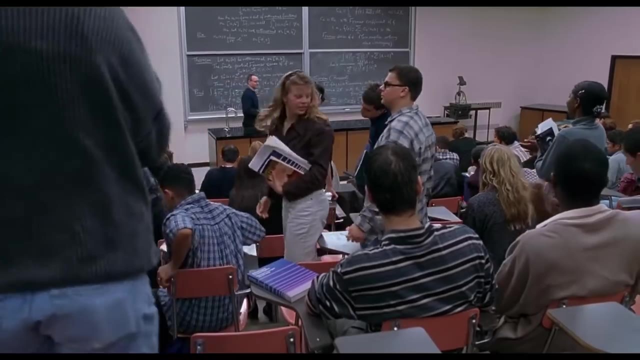 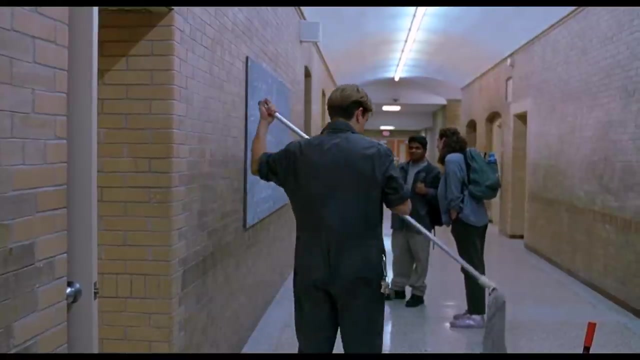 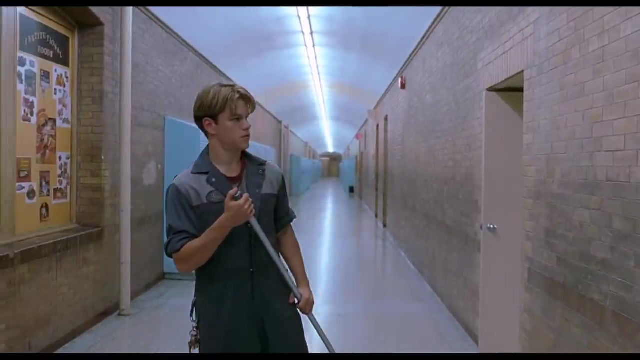 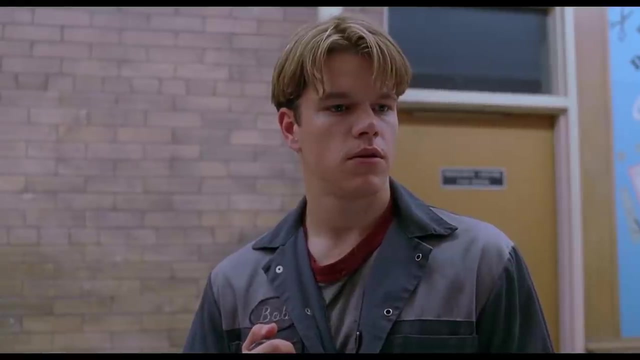 Former winners include Nobel laureates, Fields Medal winners, renowned astrophysicists and lowly MIT professors. Well, that's all. If you have any questions, I'm sure that Tom has the answers. And if you have any questions, I'm sure that Tom has the answers. 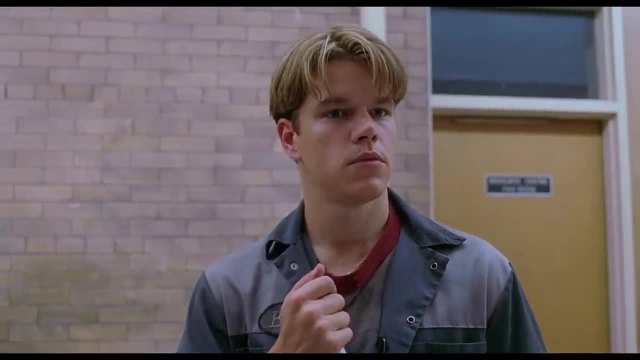 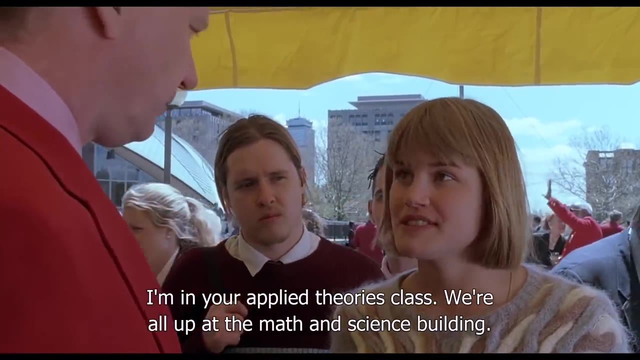 And if you have any questions, I'm sure that Tom has the answers. So I'm in your applied theories class. We're all up at the math and science building. Come here, It's Saturday, Unless you want to have a drink with me tonight. 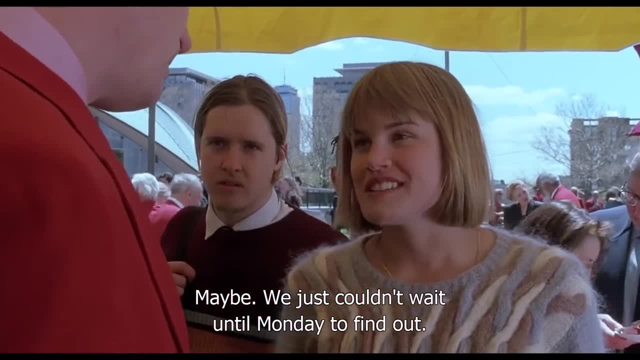 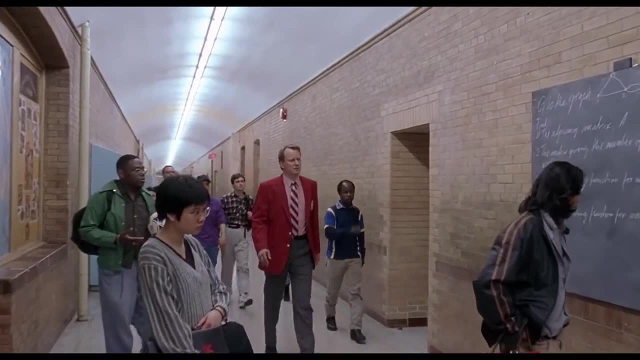 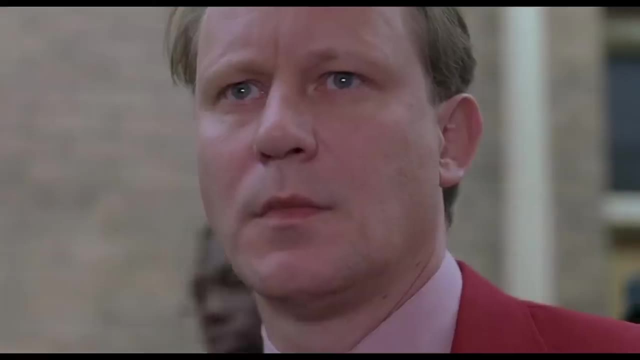 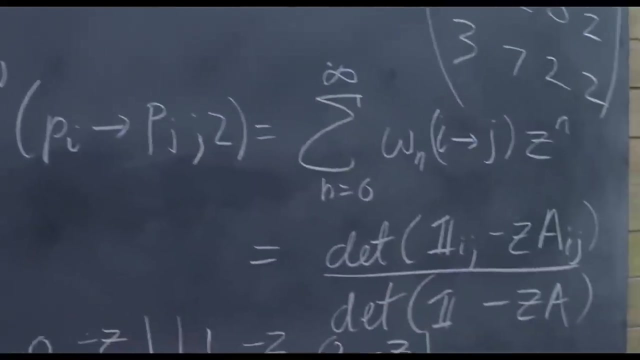 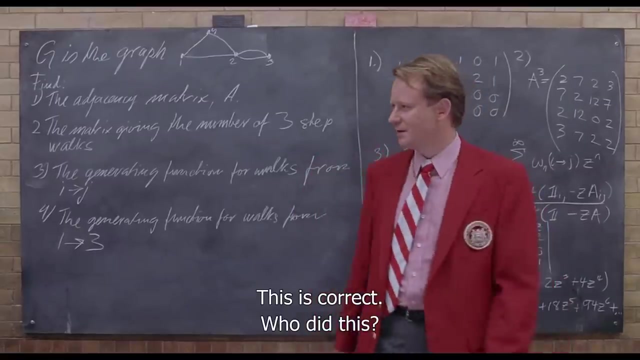 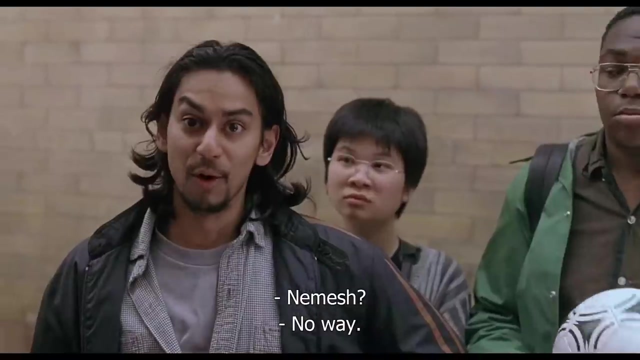 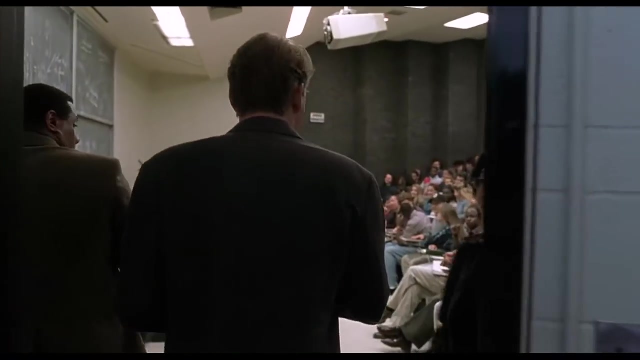 Maybe We just couldn't wait until Monday to find out. Find out what. Who proved the theorem? Who proved the theorem? This is Greg. Who did this? Jack? It wasn't me, Nimish. No way Is this my imagination, or has my class grown considerably? 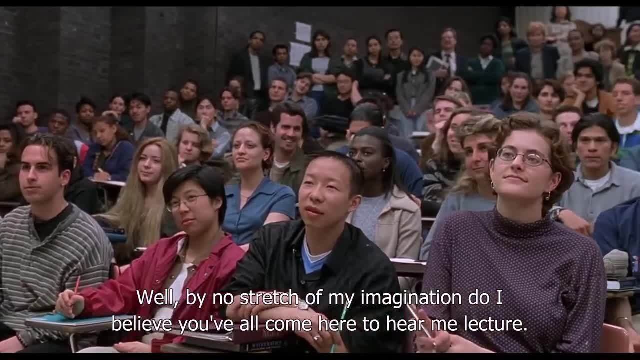 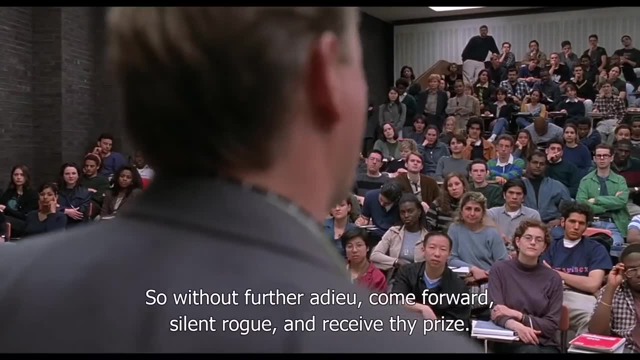 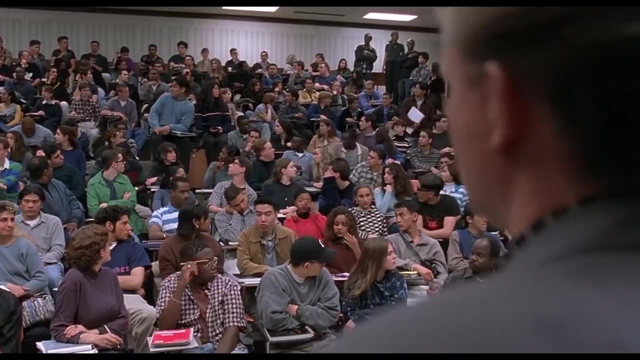 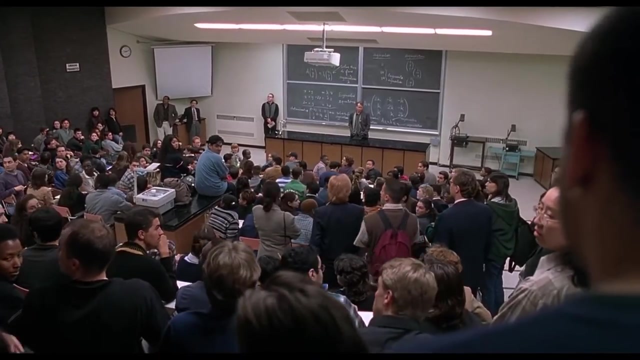 Well, by no stretch of my imagination do I believe you've all come here to hear me lecture, or rather to ascertain the identity of the mystery math magician. So, without further ado, come forward to Silent Road and receive your prize. Well, I'm sorry to disappoint my spectators. 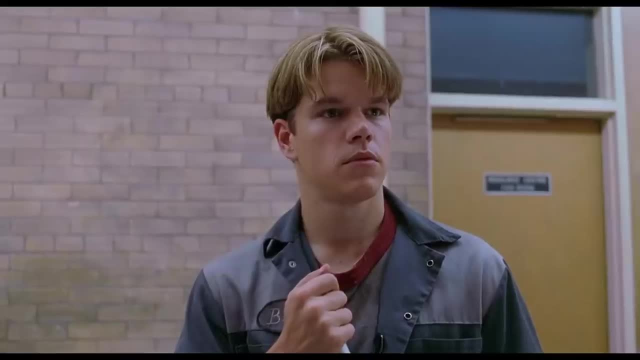 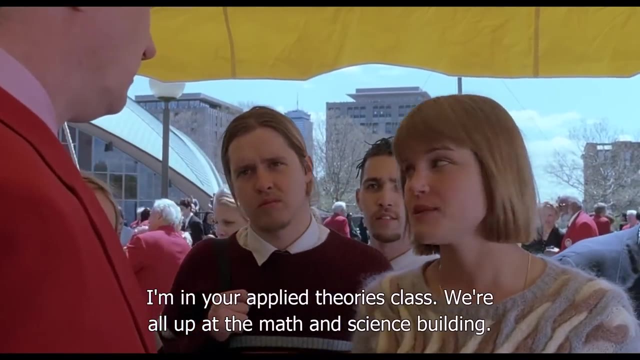 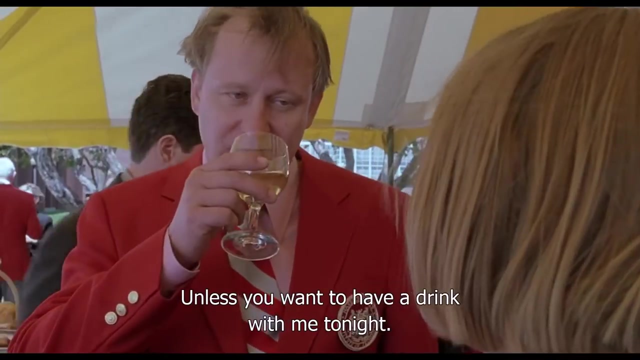 Bye, Bye, Tom. Hello, Yes, I'm in your applied theories class. We're all up at the math and science building. Come here, It's Saturday, Unless you want to have a drink with me tonight. Maybe We just couldn't wait until Monday to find out. 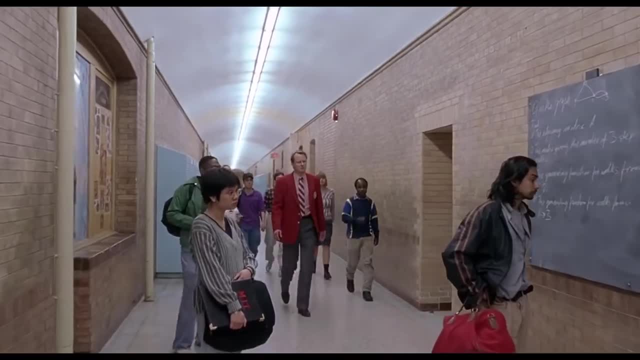 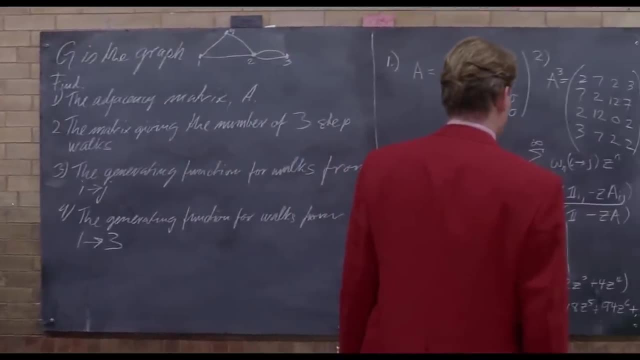 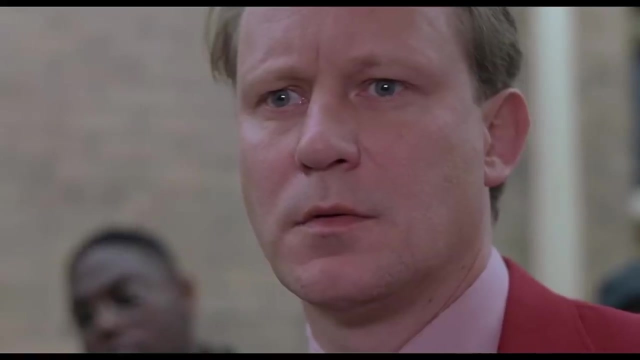 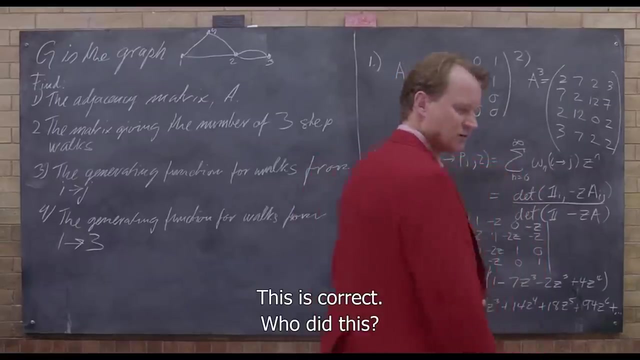 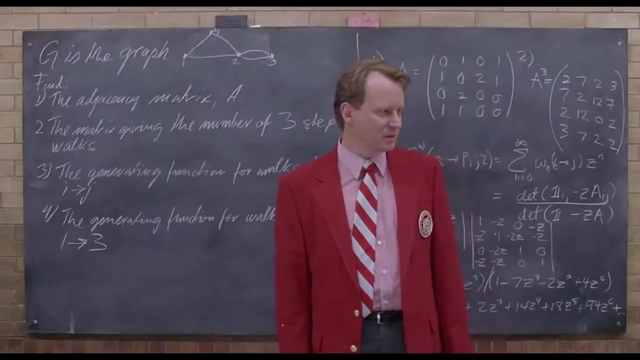 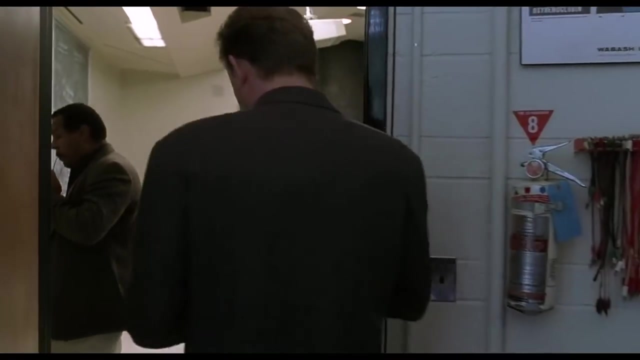 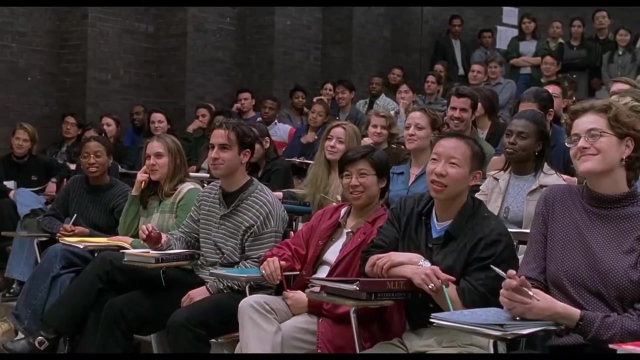 Who proved the theorem? This is Greg. Who did this, Jack? It wasn't me, Nimish. No way Is this my imagination, or has my class grown considerably Well? by no stretch of my imagination do I believe you've all come here to hear me lecture. 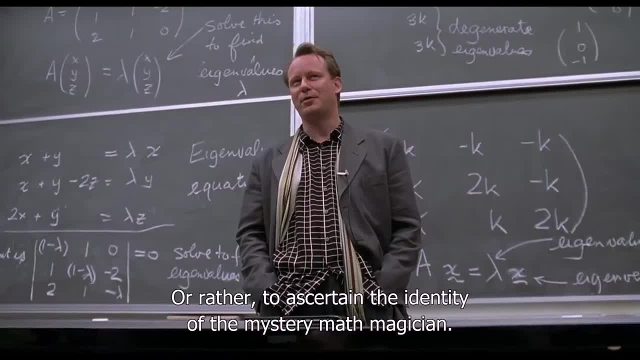 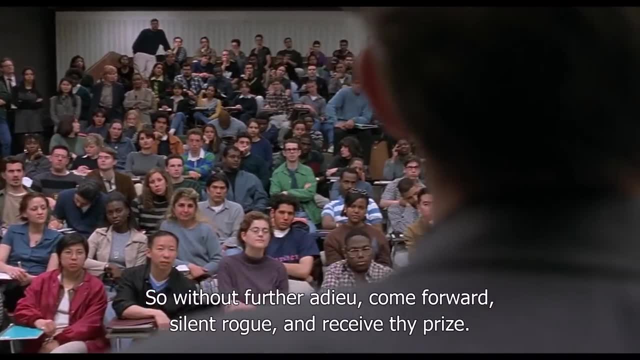 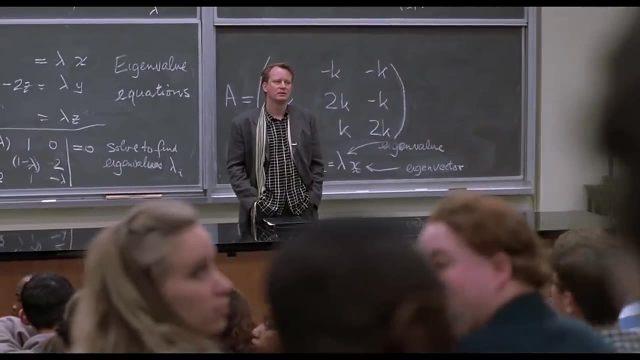 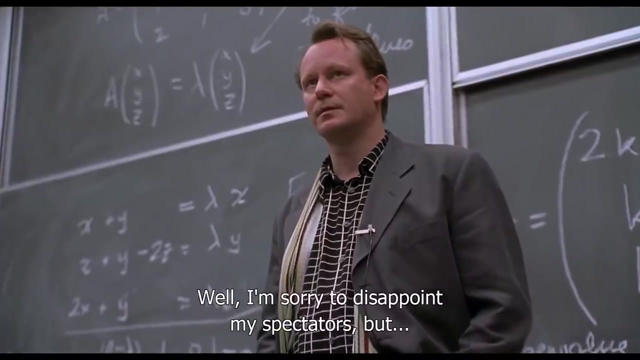 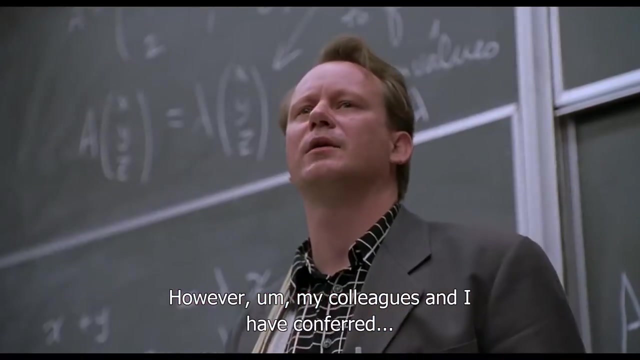 or rather to ascertain the identity of the mystery math magician. So, without further ado, come forward to Silent Road and receive your prize. Well, I'm sorry to disappoint my spectators, but it seems there will be no unmasking here today. However, my colleagues and I have conferred 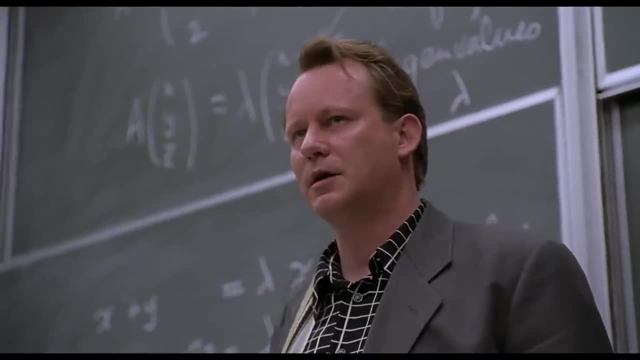 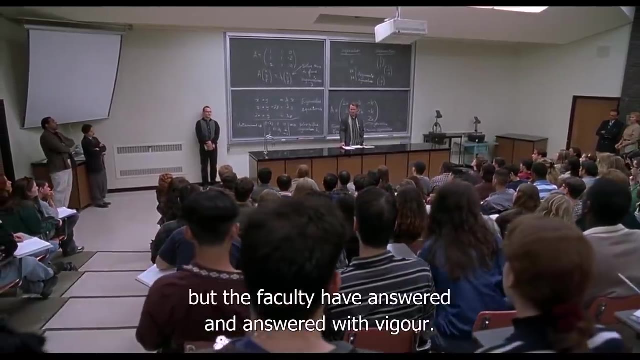 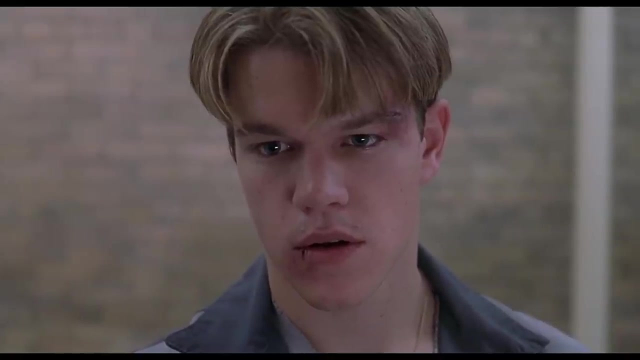 and there is a problem on the board right now that took us more than two years to prove. So let this be said, The gauntlet has been thrown down, but the faculty have answered, and answered with vigor. Very simple transformation on bifurcation. 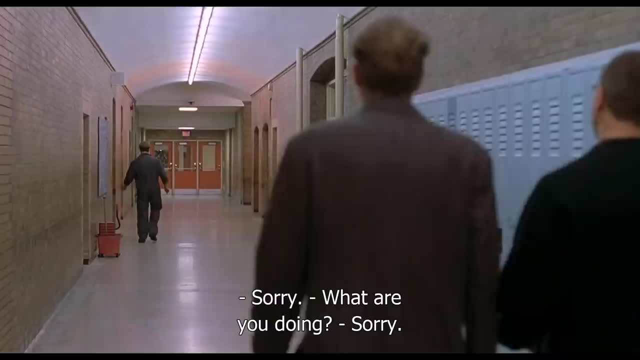 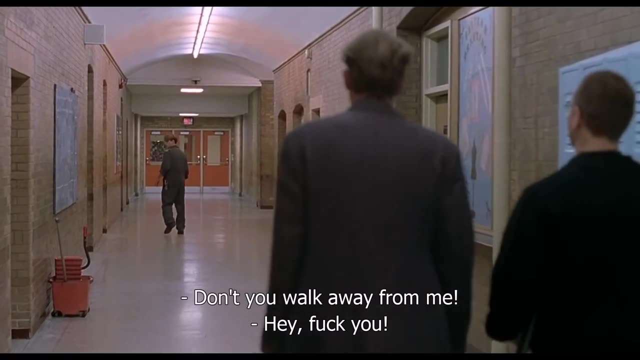 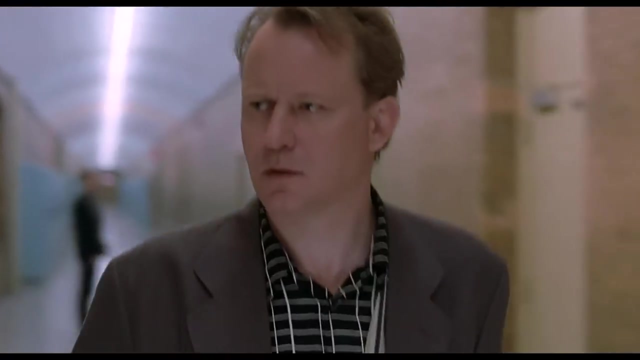 Sorry, What do you do? Sorry, That's people's work. You get your feet here, Don't you walk away from me? Hey, fuck you. Oh, you're a clever one. What's your name?